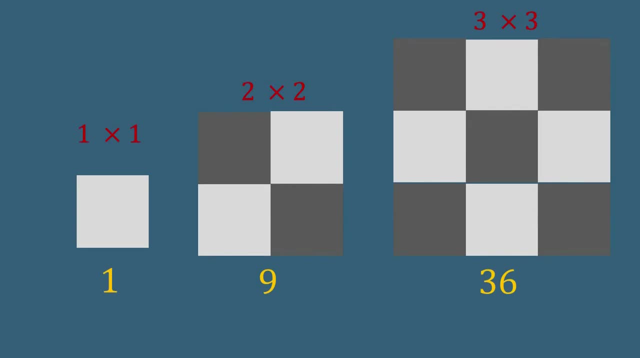 24.. and count the rectangles for the rest of the layout. Well, I have figured out the pattern. What type of pattern? Let me discuss it. In a 1 by 1 layout, the number of the rectangle is 1. that can be written as a square of 1.. On 2 by 2 layout, the number 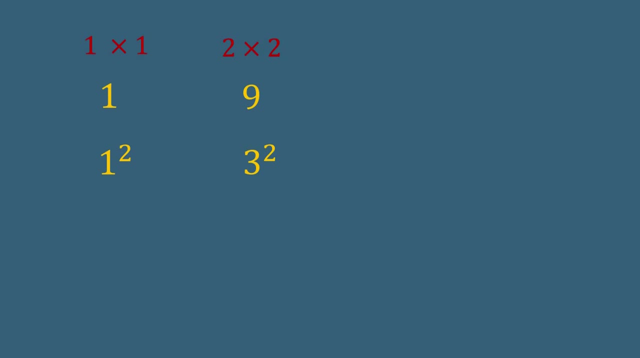 of rectangles is 9. that can be written as a square of 3, and on 3 by 3 layout, the number of rectangles is 36. that can be written as a square of 6.. Can you guess the number of rectangles on 4 by 4 layout? Let me show you the pattern: The 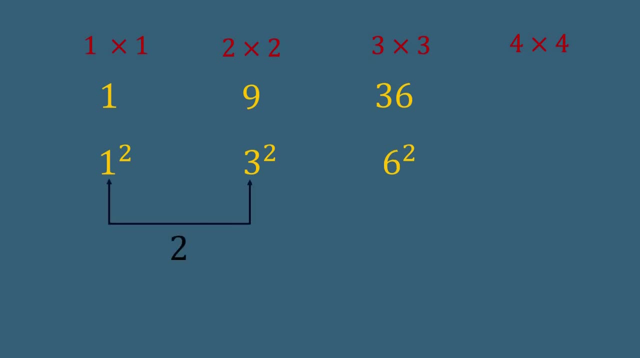 difference between the 3 and 1 is 2.. The difference between the 6 and the 3 is 3.. Now you can guess the value of X If we follow the order of difference, that is, 2,, 3, the next should be 4.. I mean, the difference between X and 6 should be 4. 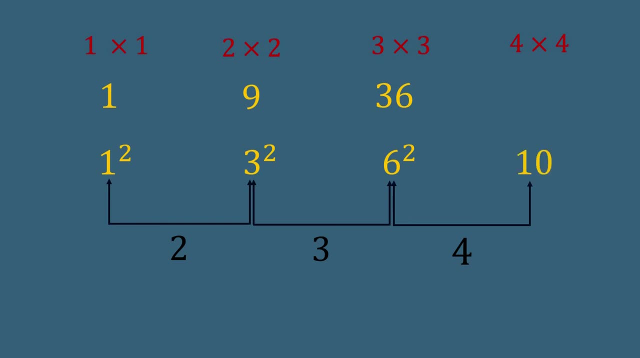 and results in the value of X should be 4.. 10. then the number of rectangles on 4 by 4 layout is a square of 10, that is a hundred. so the number of rectangles in 4 by 4 layout is a hundred. but we want to. 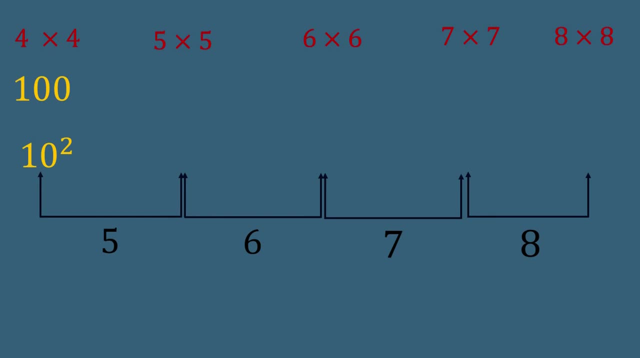 know the number of rectangles on a chessboard, which is 8 by 8 layout. for that let's continue the order of difference between layouts following the order. after 4, 5 comes and 10 plus 5 is 15, the number of rectangles in 5 by 5. 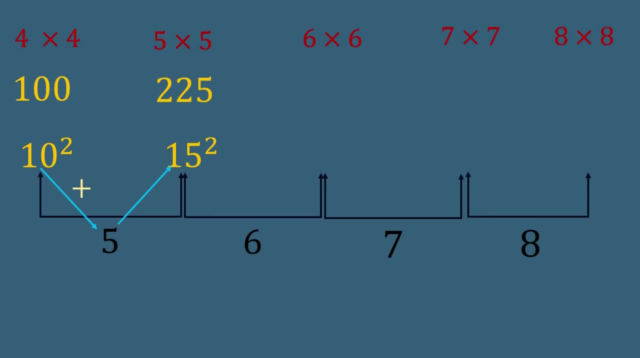 layout is a square of 15, that is 225. now, 15 plus 6 is equal to 21. the number of rectangle on 6 by 6 layout is square of 21, that is 441. 21 plus 7 is 28, so the. 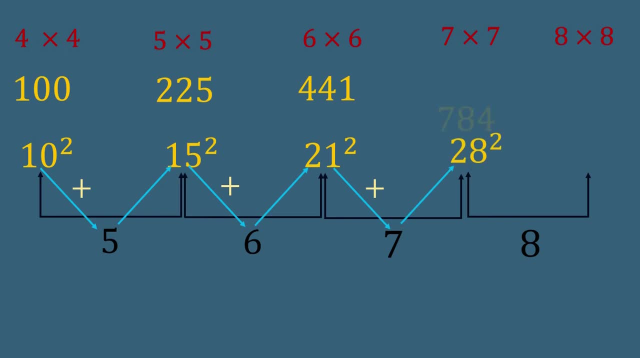 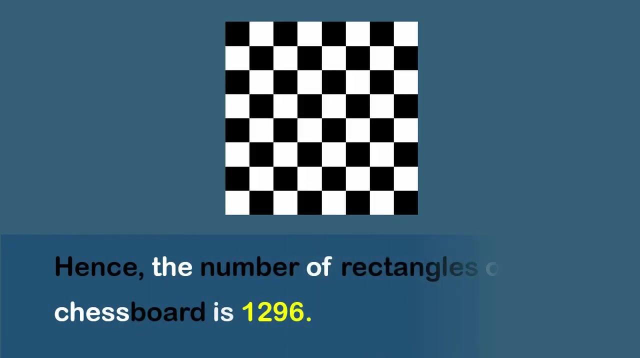 number of rectangles on 7 by 7 layout is 341,, 242 and 343. the number of rectangles on 8 over 8 layout is finally, 28 plus 8 results in 36, and the number of rectangles in 8 by 8 layout is 2996. hence the number of rectangles on a.